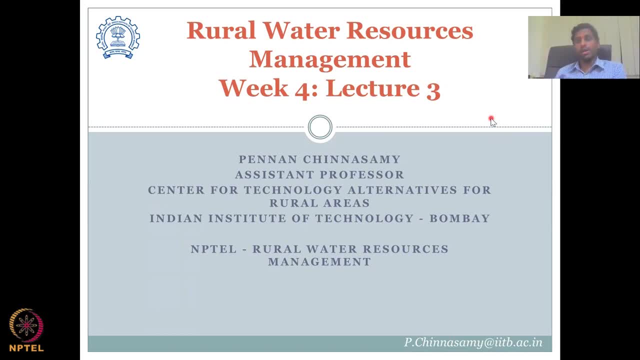 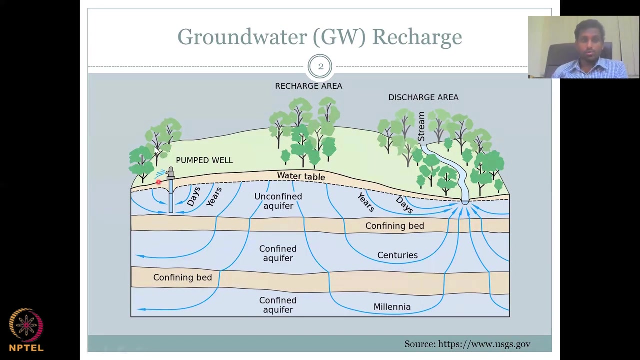 and then discharged or pumped out, used, etc. So now you have a better idea of managing the groundwater resource. if we know about the recharge and discharge, Let's start with groundwater recharge. So the recharge area which you see on the top of the land is going to be the predominant. 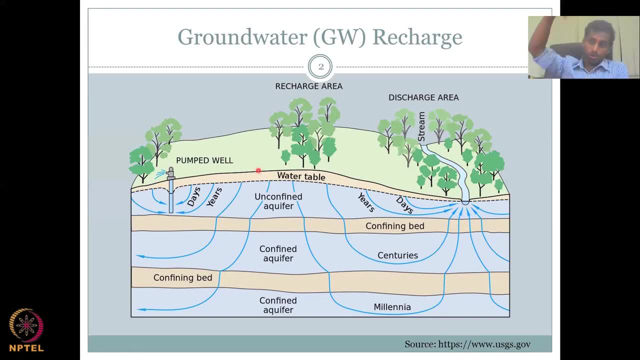 phase where you have water coming in. Water comes through streams and rivers, but it's much less compared to precipitation-induced groundwater recharge. Visualize yourself as a water droplet. You'll come, infiltrate and then get into the first unsaturated, then saturated zone. Once you get into the saturated zone and you have 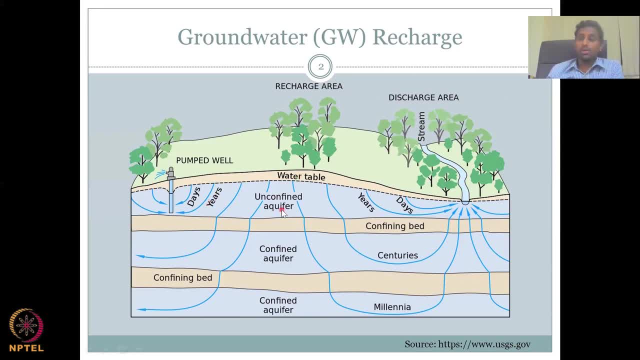 a confining bed, it becomes an unconfined aquifer. Remember, I was saying that you don't just have to have one confined aquifer. there can be multiple, But you can only have one unconfined aquifer. There cannot be an unconfined aquifer suddenly after a confined aquifer. 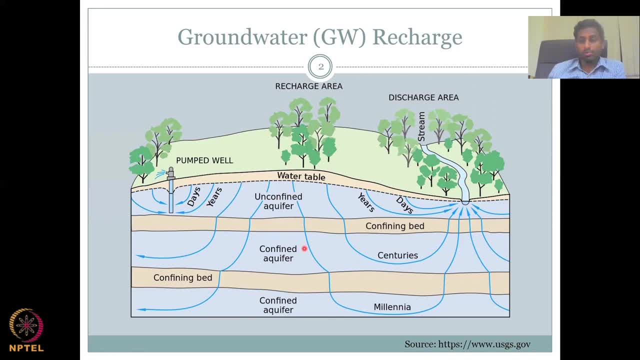 So only when you dig it up. yeah, if you dig up a well and you have open aquifers, you'll see open water coming in. then it is unconfined, But you would call it as an aquifer because it is a longer time and space. 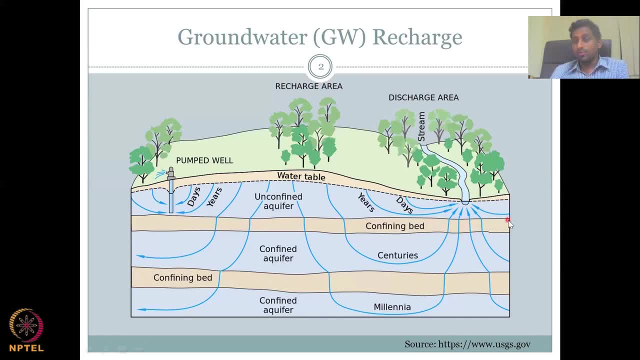 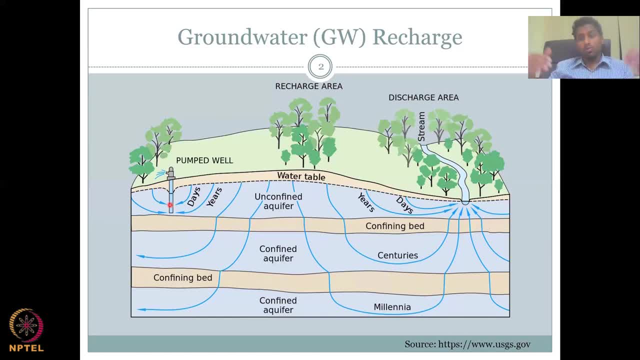 You will see it coming into your pump well. So the well is where water gets stored. You will see the water level rise. So you know that recharge is happening because of the rainfall. If you put a well here, you can also monitor the level rise when water is flowing in the 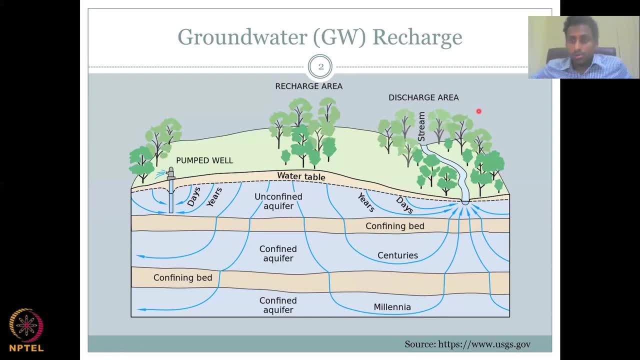 stream. So that also gives you an idea about water level rise due to recharge from water from the spring. Spring Springs can also give water to spring. So coming back, let's look at this angle only for now. So rainfall comes in, recharges your groundwater and flows into your wells. 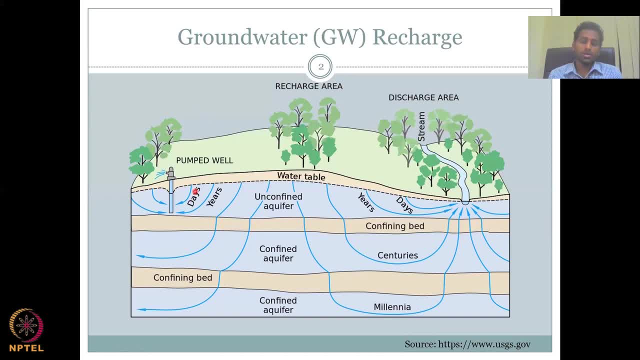 It takes a couple of days, anywhere from a day to a week. Then you have further away. Further away, water can come due to precipitation infiltration and then go into your well, which will take years, Depending where your aquifer is stored, depending where the point of water access is there. 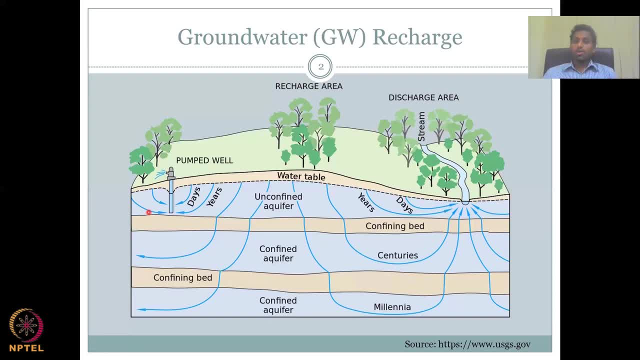 the water would have to move a long term, a long term and distance And groundwater flow is very, very slow. So please look at this: Because it is slow, it would take years. And why is it slow? Because there's a lot of obstacles on the way. 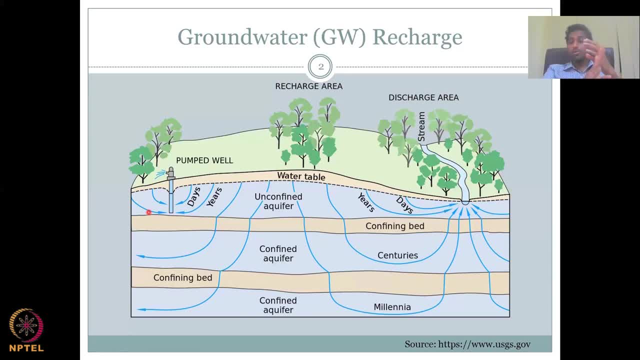 The solid materials are there, So water has to go around it, connect it through another pore, those kind of things. And if there's already water, it's less. With the high potential, I'm saying, then water movements are balanced out. 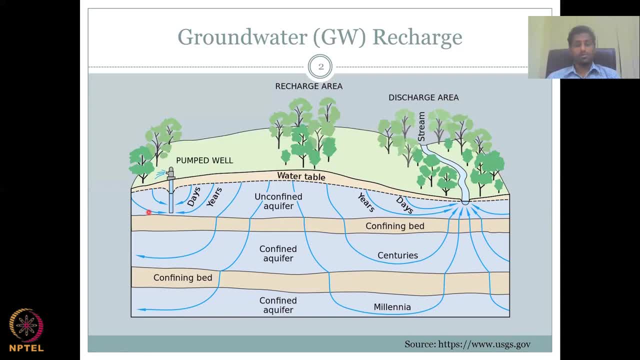 So it takes anywhere from years, okay, in the unconfined aquifer, So anywhere you can start from a days to years. For example, in the Ganges basin you could see it within a days that the wells start to recharge when there's good water flowing in the river and also good rainfall. 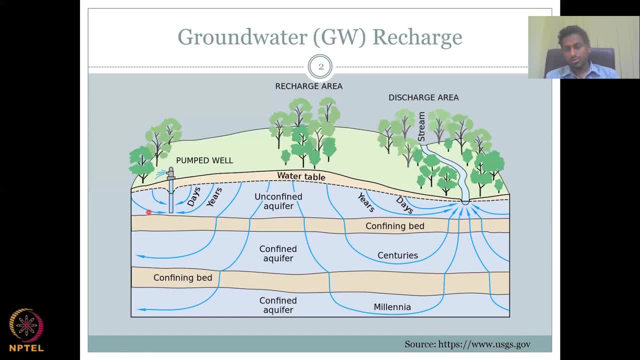 It may not be the same in central India. It would take some more days to see the groundwater rising up, And then some somewhere in the drier regions. you would see years. okay, Let's get into the confined unit Now. here comes the lag, the delay. 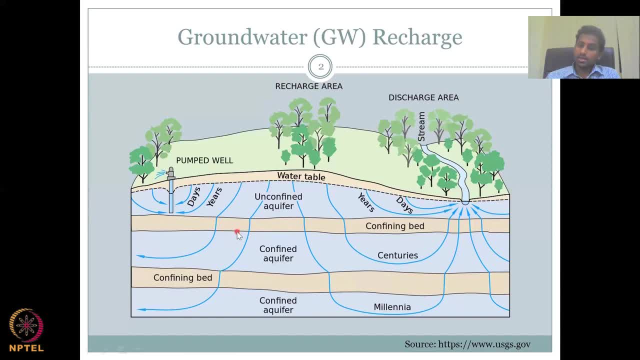 So water can come, but when it sees the confining bed or impervious bed it cannot straightly come into and recharge. It takes long, long time- okay long time- the water has to sit on top of the surface, slowly infiltrate. 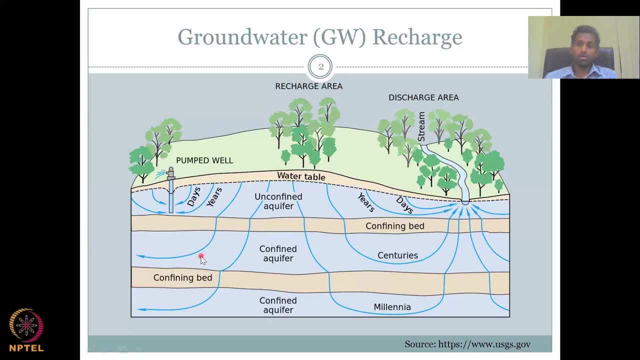 Or water comes from a longer distance. okay, Distance can also increase the time the water takes to come into the aquifer. So now I'm looking at confined aquifer one. this is confined aquifer two. okay, For the confined aquifer, water can come from a very far distance and then move slowly, slowly, slowly into this aquifer. 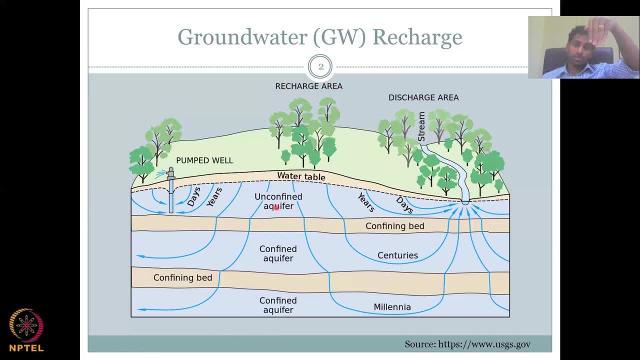 Or water can come from the unconfined, but stay there for a long time and then infiltrate, Penetrate through the impervious layer. Whatever, it is impervious, there's still some leaks. okay, It's not 100% impervious layer. 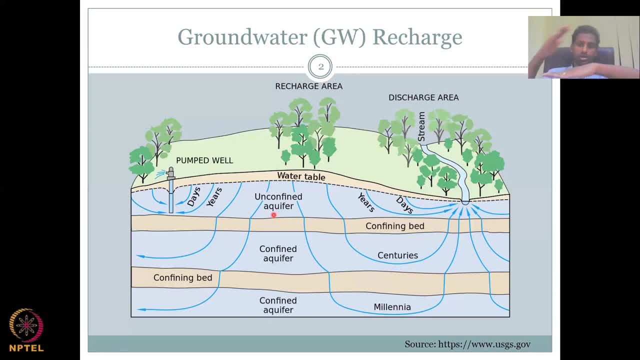 It's not a steel put so that it just stops your water, It's a stone, It's a rock, So some weathering can happen, So water can move through. okay, And that takes centuries, hundreds of years for the water to come there. 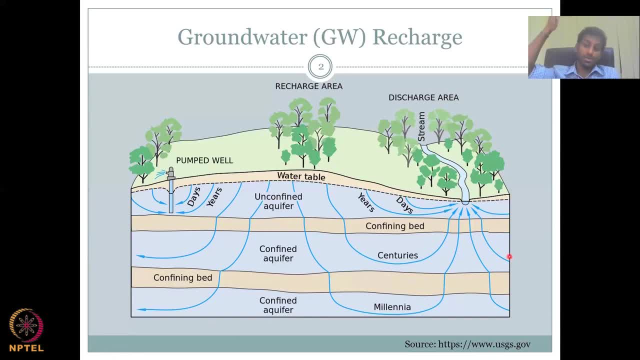 So that is how long water takes from the surface. Okay, So water takes from the surface to come into that aquifer. Then you have the next confined aquifer, which is at a much lower depth And it has two confining units to jump. 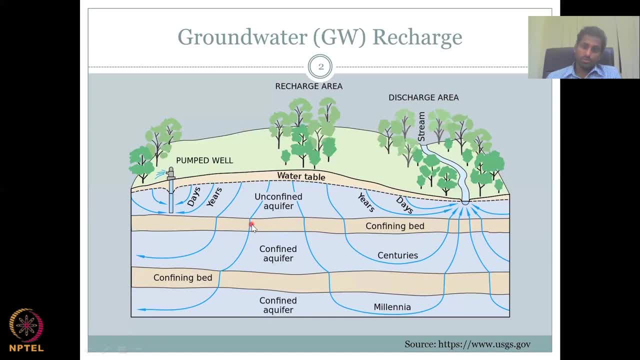 So water has to come. go to the unconfined aquifer. then jump your confining bed, which means infiltrate. come into the confined aquifer. Here it can move faster because it has four spaces, so it can move much faster. 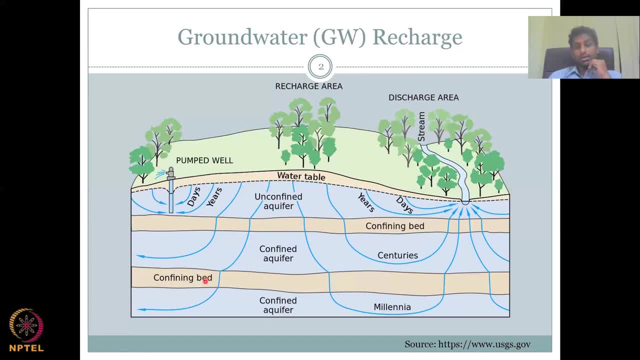 And then it goes into the confining bed again. Now again it has to infiltrate, wait, slow down and then get into the confined aquifer. This takes a millennia, which means a thousand years. So see how the same water can go from days recharge to years recharge, and also from centuries to millennia. 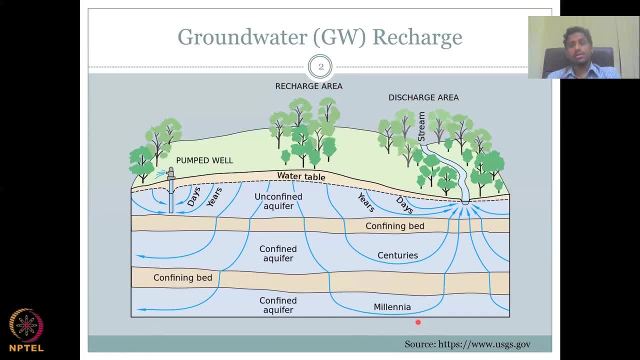 So it is very important to understand the time groundwater takes to recharge And this, I hope, has clarified your question. I hope has clarified to understand that part so that we can put better rules and regulations for using the water. For example, if you have a pump in the unconfined aquifer, you're okay that, even if you dry it out. 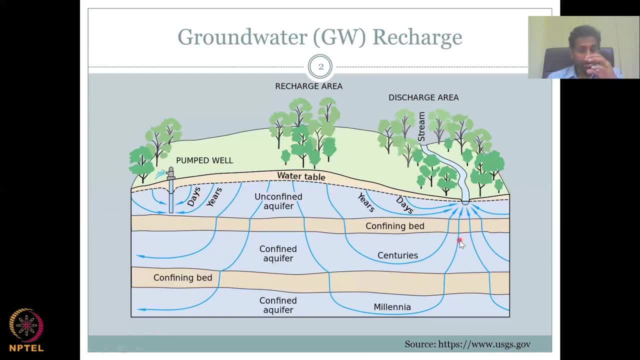 For example, I'm pumping all the water out And after rain the water can be recharged in a day, couple of days, a week or max by years. Within one or two years, good rainfall water levels will come up. 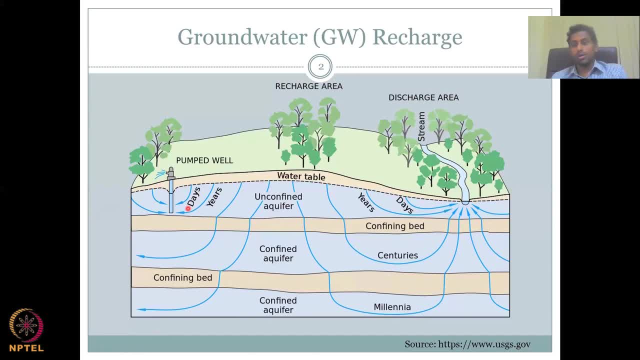 So if you see, right now All the areas in India are getting good rainfall, So all the groundwater levels are recording high, So some wells are there. But if your well is in the confined aquifer one and you pump out all the water, 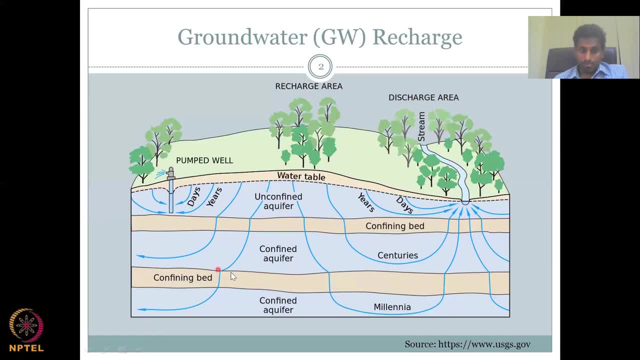 So for it to refill again, for it to come back to the original level, it could take centuries, Not one but multiple centuries. So you are actually taking your future generation water, Or the water that has been given to you by past generations for you to save and to use wisely. 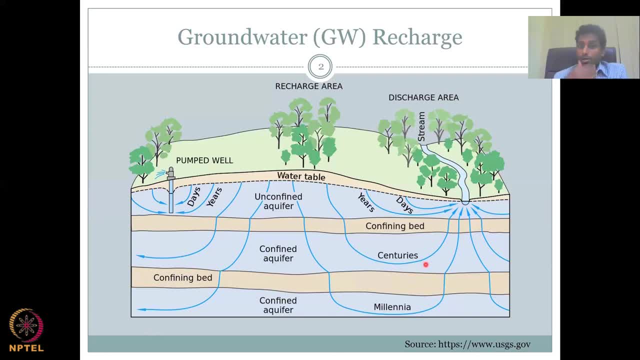 If you pull it out, within ten years- five years, which is happening right now due to agricultural expansion- People doing two rotation crops, three rotation crops, in an area where only one rotation of a crop should be done, If you're too much using the water, groundwater resource. 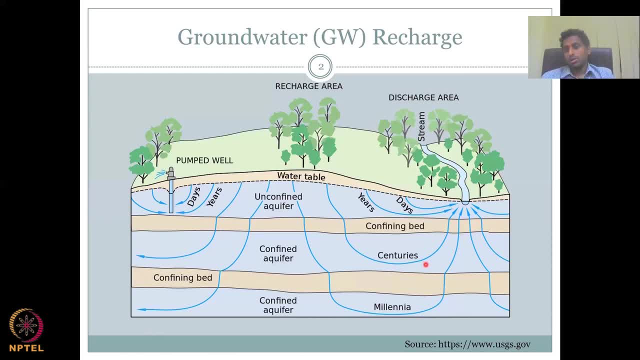 Actually are taking from the past and the future groundwater demand. So it is as much more important to conserve the groundwater Now coming if you have a well so deep. So in some parts in the drier regions you can see wells going to 400 feet, 600 feet. 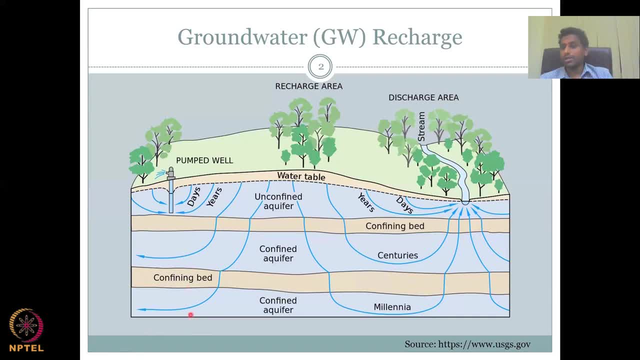 What does that mean? So you are actually tapping the very deep confined units. Once you take the water out, it's gone. You're not going to wait for another thousand years to come, And that is where people abandon the wells. Same here. 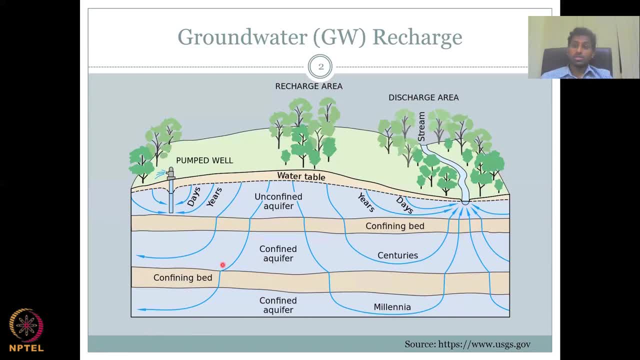 If you have a well here, the water is taken out and you see, you wait for a couple of years. the water doesn't come. People just move on. They say, okay, it's abandoned. well, I'm going to go for another area and put another well. 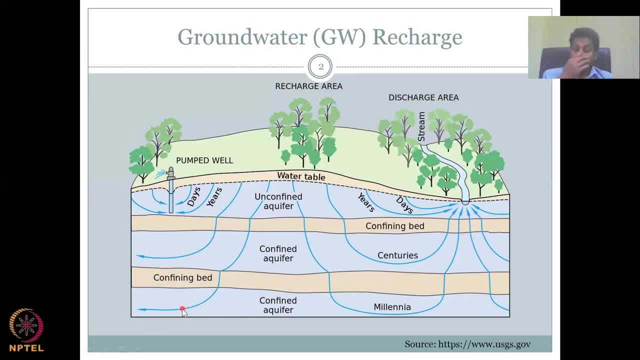 Same here: If you pump out all the water, then it goes up, But that is not sustainable, right? Because you use some water which was there for over a century. So it is as and more important to conserve groundwater. I hope this actually brings in a lot of sensitization on using of groundwater, understanding how deep your well is. 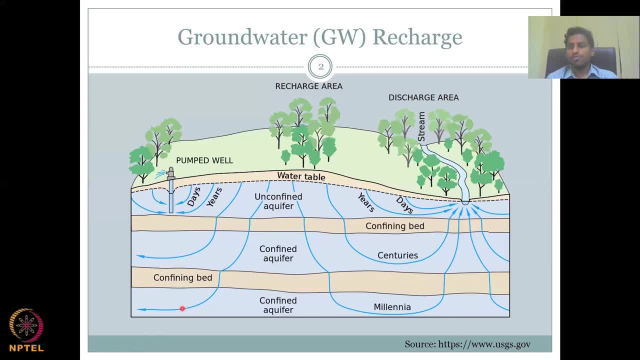 So your depth of the well can actually give you a rough estimate of your aquifer. So if you're tapping groundwater, let's say within 30 meters, you're well and good. You say, okay, 13 meters, it should be an unconfined aquifer. 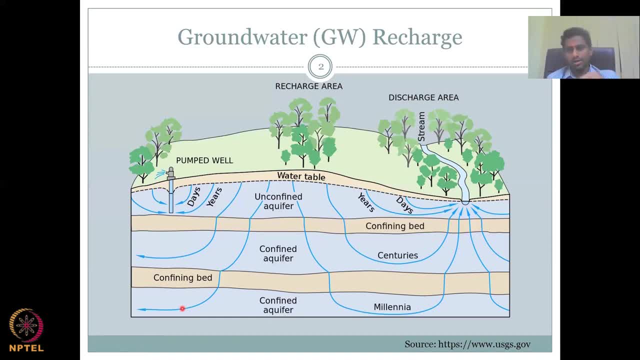 Technically, the soil profile is there, Water can come in- Okay, well and good, And this without talking about pollution. But then when you have your confined aquifer, when the well is further deepened, when you push your bore well deeper, then you're taking water from a deeper confined unit. 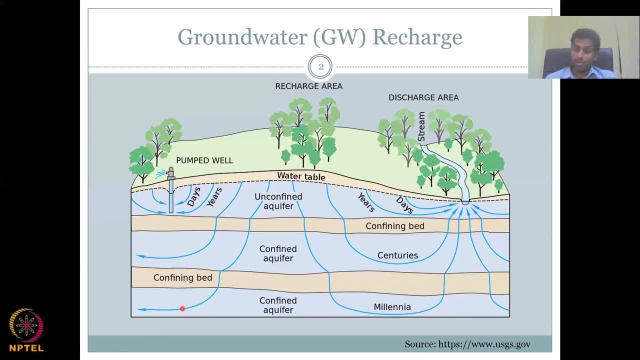 And once your water level is coming down, which means you're using the water and the water is running out- it is an alarming well. Alarming well That you need to start recharging, start doing some other practice, Start doing some other practices to bring the water well back to a sustainable level. 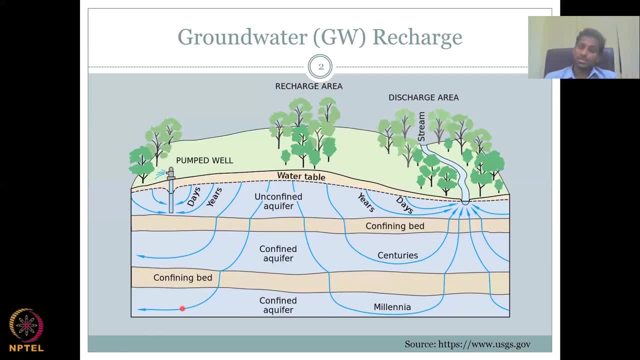 Okay, So please understand that it is not the same recharge rate across. It differs, and it differs at a big, massive difference: Years, days, millennia, centuries. So you should not be using what water you took for a century to recharge within a year or two. 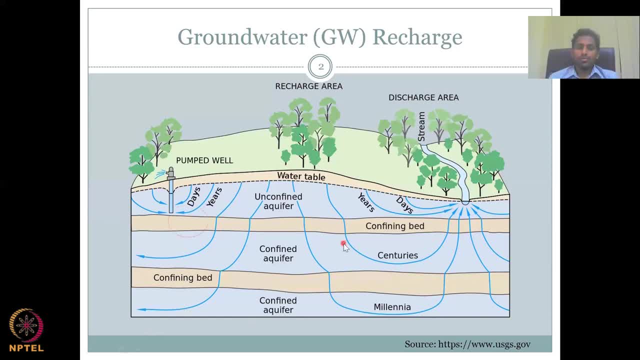 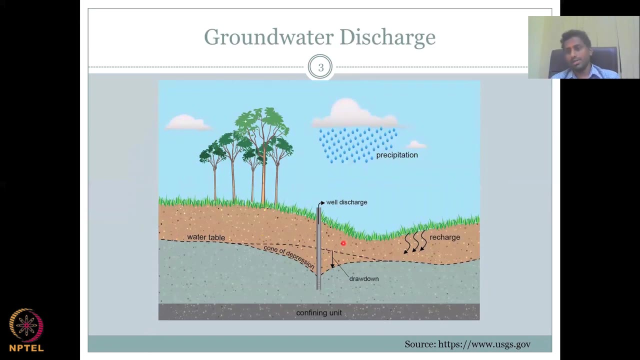 So it has to be conserved. Moving on, you can have days and years also in the same unconfined unit, But, more importantly, conserving the centuries and millennia water is important Groundwater discharge. Now we are in a groundwater discharge slide where we talk about pumping or taking out water from the groundwater aquifer. 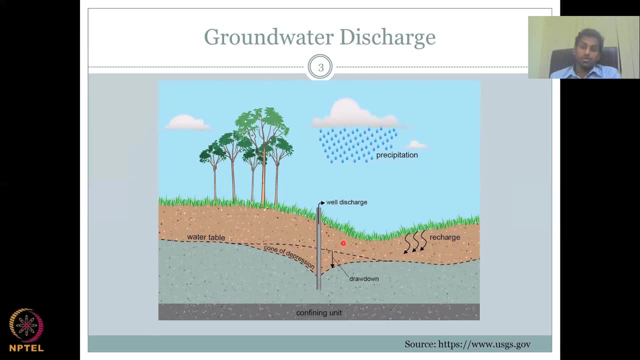 And that act is called discharge. Discharge can be of two types. One is forced discharge, where you put a pump and you pull it out to energy or manual labor etc. Or by naturally groundwater can discharge into a system or out of the system. 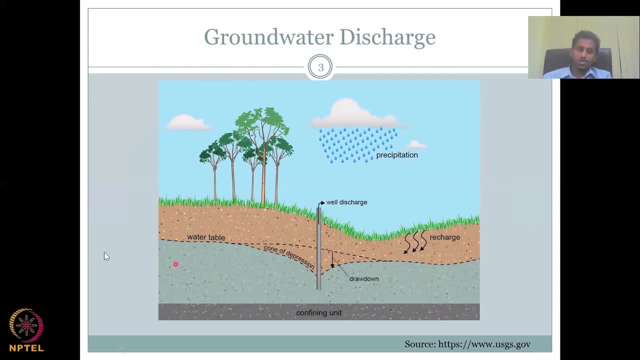 Your precipitation happens, Your recharge happens, You have your aquifer formed, Your water table is there. Then you start to pull water out through your pump for agriculture, For domestic use, For livelihoods, industry, Be it any use you want, But you are pulling it down. 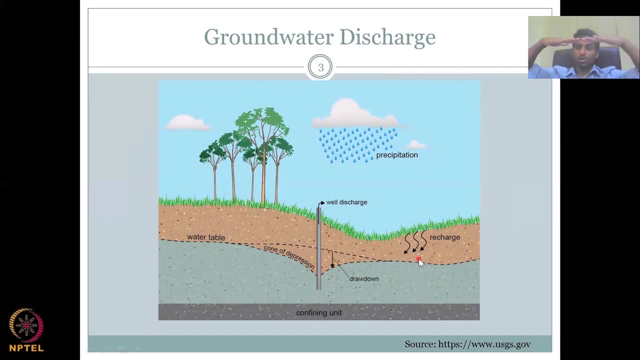 So once you pull you can see that the water table is not the same And water table doesn't go down like this. First it goes as a cone of depression, Which means around the radial area of the well. suddenly the water level will come down. 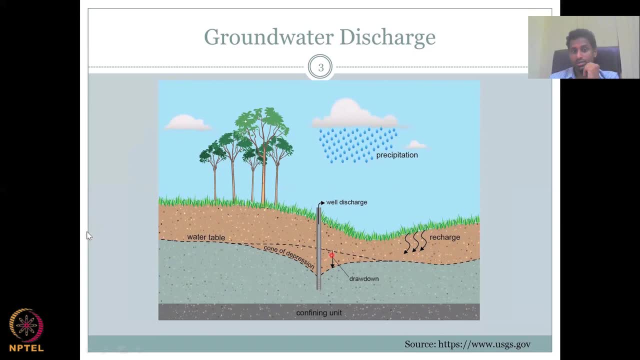 Because all the recharge that was happening evenly, evenly has created an even water table. But your localized pumping is pumping at one point. So even though there is recharge happening on the sides, because of this pumping, all the water will go in as a cone of depression. 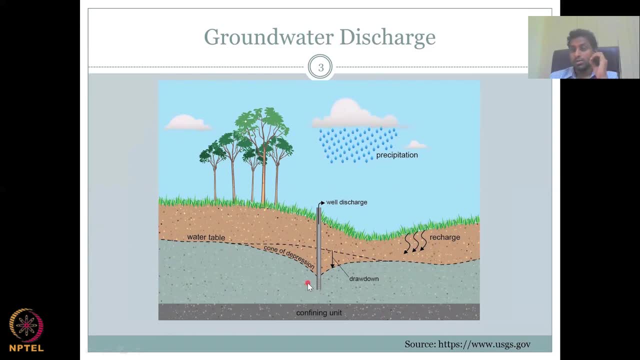 So once you have the cone of depression, this is the worst part. If you have a cone of depression, then the water table, which was almost stationary because of the same potential, now starts to flow to your wells, So you're not actually pulling water from a different distance. 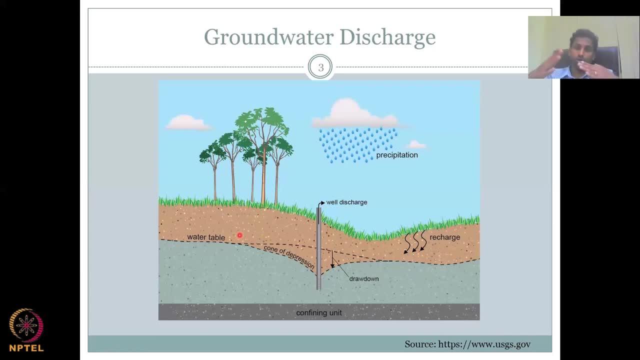 But by the act of pulling you create a cone of depression. And once you create a cone of depression, there is a potential difference between this water table and the water table here. So the water table here and the cone of depression here, there is a potential difference. 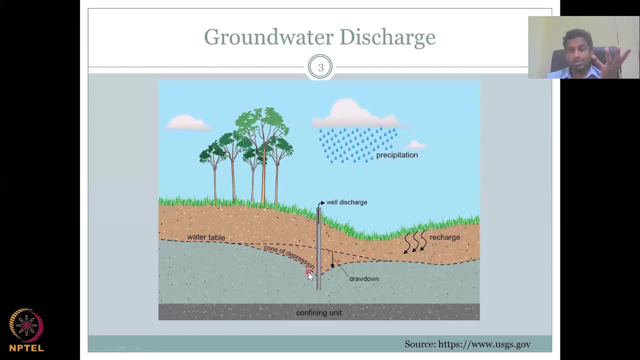 High potential, low potential, And because of that water will go naturally to the well, So you don't have to pump with more energy. So this is where farmers are losing it. They think, Sir, if it is recharging faster as I pump, then there is a lot of water. 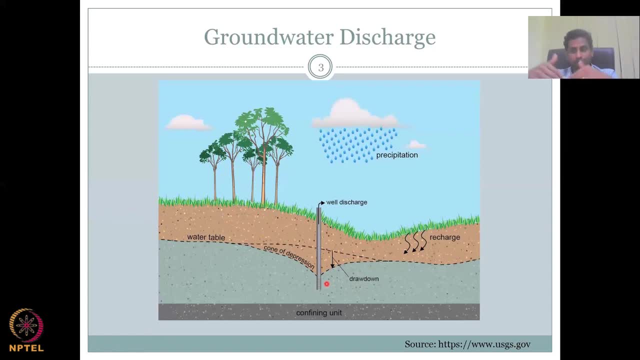 No, Because the cone of depression is forcing the water to come in. Think about: you have a glass of water, You're putting a straw and you're taking water out. Initially you have to have less energy, But when you go down further, you have to spend more energy to bring the water out. 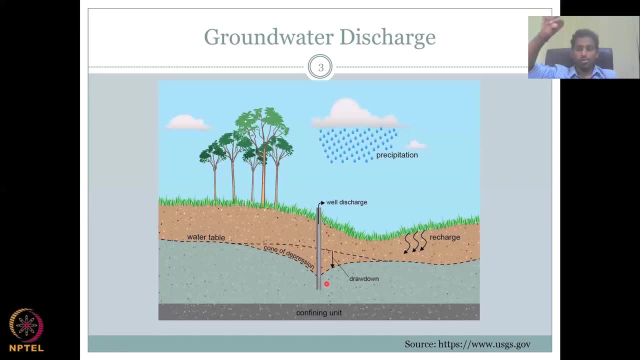 Because there's no water coming in. If it is pouring in more and more water, then it's the same, But here because there is a potential of a cone of depression, because water is not, It's not a river underneath. You still have soil, materials in the aquifer. 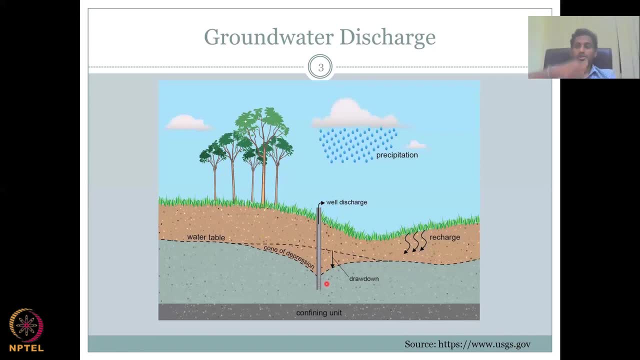 So that is where the cone of depression forms. If it is a river you pull, then the whole water table will go like this: Just visualize you drinking water from a straw in a cup. If you drink, it goes like this: the water level. 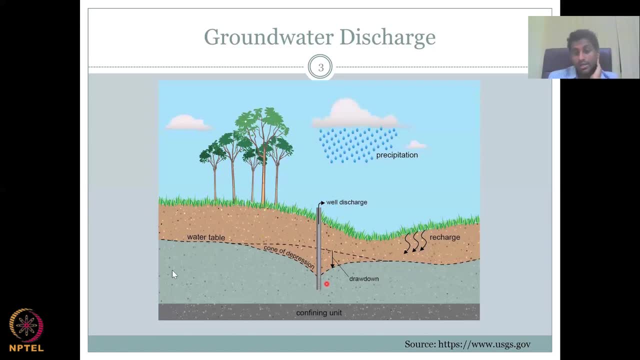 It doesn't go like a cone of depression. It is purely water Here. because of your sediments, solid materials, only the water is released. That's why you see it's still brown. After you take the water out, it becomes brown. 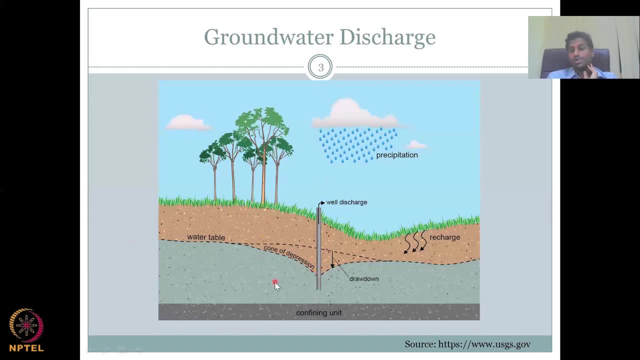 Just no water. So the cone of depression is kind of concerning because it actually pulls water from around your area into the well for easy access of your water. So the water level doesn't increase but the water coming into the well increases. 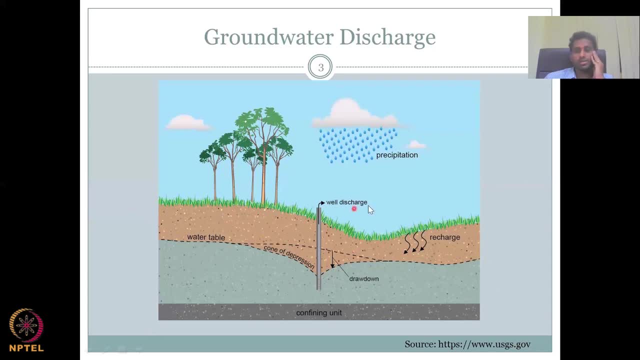 And you keep on pumping and discharging it. So here's where, if your pumping cost is very low, if it is supplied by an alternative energy which is very low, for example solar pumps and other things- What can happen is if you do not have concern of pumping for the energy, then too much water can be used. 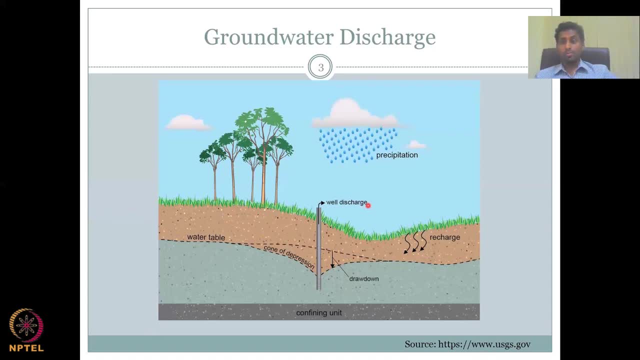 Too much water can be extracted, So it's always important to meter your pumps, Understand how much water you're using, Only use what water you need for your crops and then stop. Otherwise, this cone of depression will go bigger and bigger. 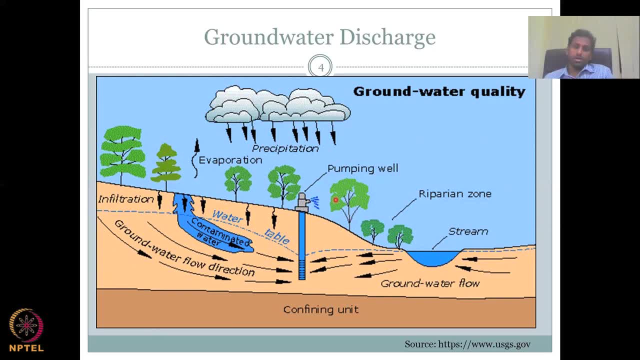 Another groundwater discharge diagram. Again, you can pull water from your groundwater aquifer And also you could reverse the sign of your stream network. So initially the stream was getting groundwater from here, So it was a gaining stream. But because you're pulling and because of the cone of depression, you have been pulling the water from the stream, which is a surface body, into the ground. 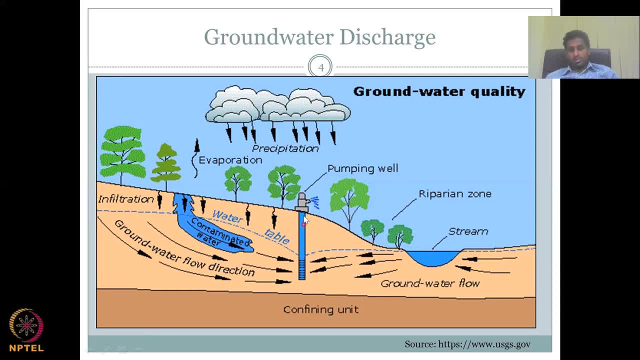 Then it becomes a groundwater And then back into the well. So the well is now pumping it out. So the groundwater flow diagram is given. Infiltration happens. Leave the contamination. That's not in this course. But evaporation losses etc. etc. 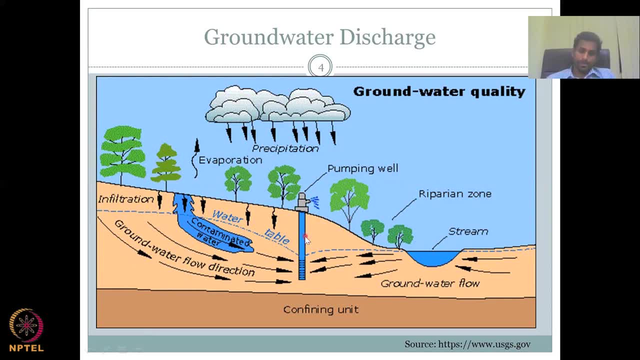 Water comes in, Goes into your pump because of your pumping, And then you have a cone of depression And because of that depression, a high potential- low potential gradient is formed And the volume of water is now pulled. So where does the water quality come into the picture? 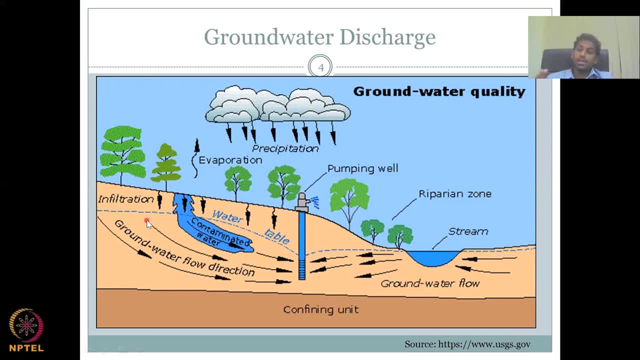 Because if you have a contaminated source, for example, a landfill or a septic tank which is broken, and a lot of waste- solid waste- is here And it is standing there Because of the high water potential. But when you pump too much and the cone of depression is formed, then you actually start pulling the contaminated water which was initially not moving. 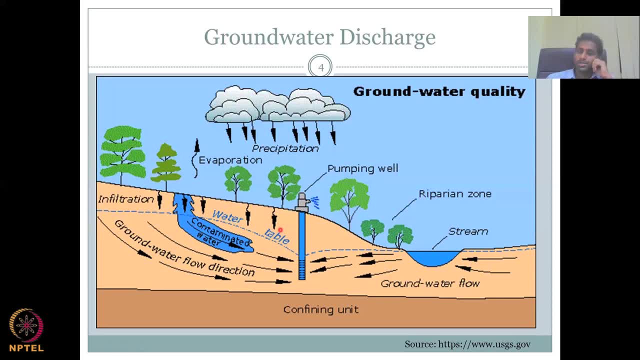 So it is always important not to put groundwater wells near contaminated sites, sewage lines and then over pump it. So if you over pump it, the cone of depression forms And even though the polluted water did not want to move initially, because of this cone of depression it starts to move. 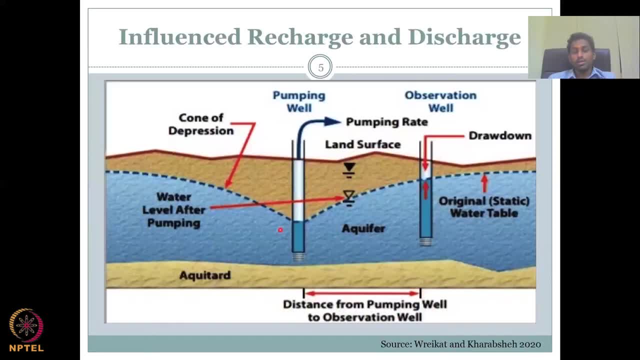 Then you have an influence recharge and influence discharge. So what we saw in the initial stage is: if you just pump and the water table comes down, there is no influenced discharge. But when a cone of depression is formed, there is an influence discharge. 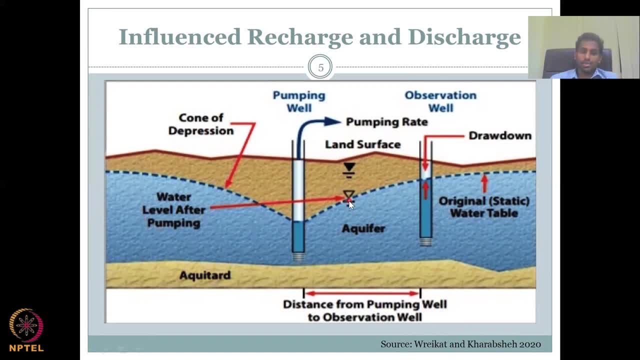 So water level after pumping is here. It recovers, So water recovers, but still the cone of depression is there And your initial water level was here, But because you pulled water out, you could see. So now let us take two wells in tandem. 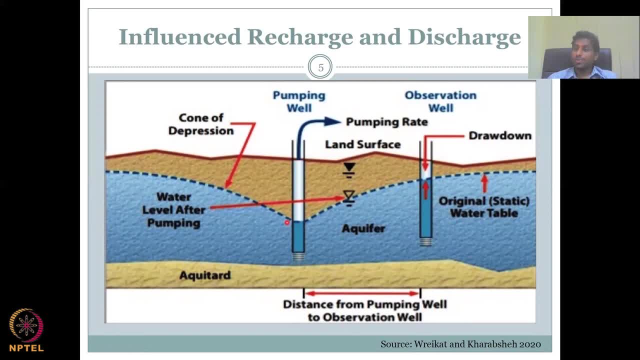 And this is where the well monitoring I was talking about, of representative mass, etc. etc. So you have a well here. Let us call it well A and then well B. Well A is used for your irrigation, for applying water to the crops. 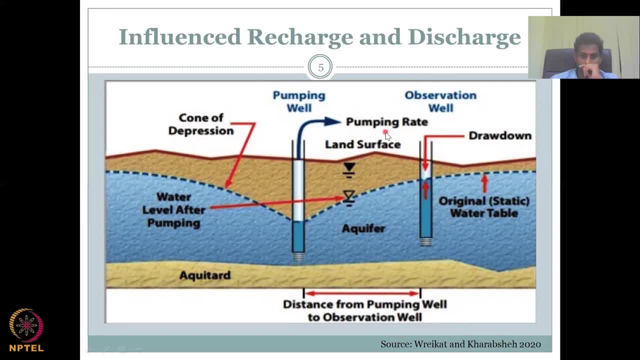 So you put a pump, you pump the water out and you apply the water. And then what happens? The water falls on the surface and you are irrigating, But meanwhile you are creating a cone of depression. There is a well B, which is a little bit farther away, and no pumping is happening. 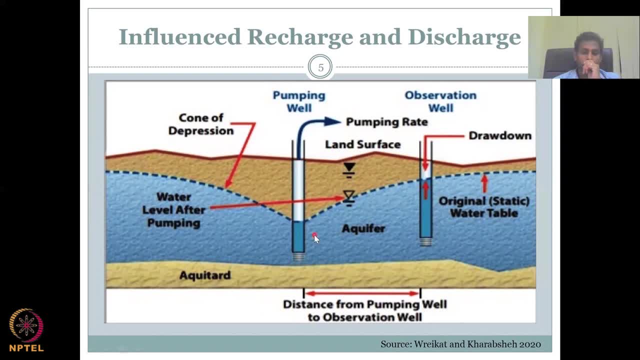 There is no pumping here. So what happens? Watch closely that when you are pumping in well A, the cone of depression is formed and the actual water level from your well B is falling. So now visualize this. So now visualize this as two farmers. 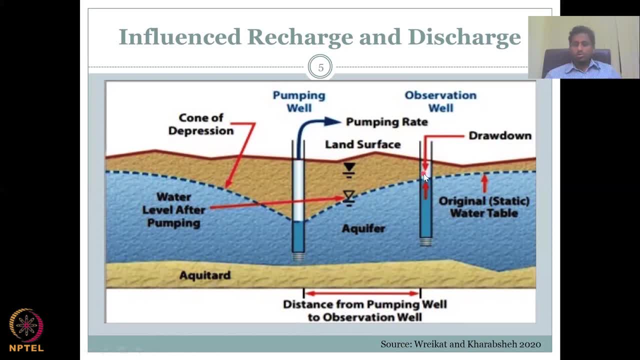 This farmer is an ethical farmer who says: no, I do not want to grow crops in the summer because there was not a good rainfall. I am not going to use groundwater. But this greedy farmer says, no, I want to use groundwater, all the groundwater, and then grow. 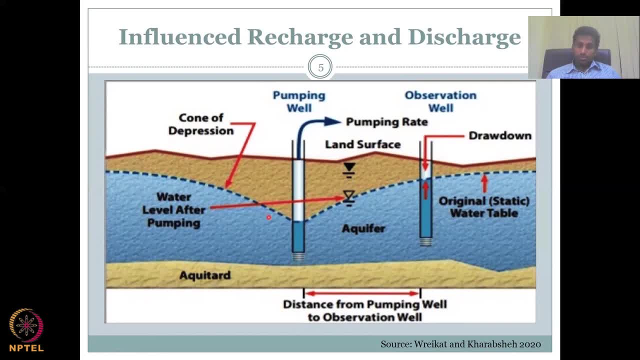 He, she, is not only using their groundwater but also the water level from here. So even though this farmer, farmer B, did not put a groundwater pump and use the water, his or her water levels is also coming down. So here is where a communal source, a water which was for the community, for general public, has become one person's property. 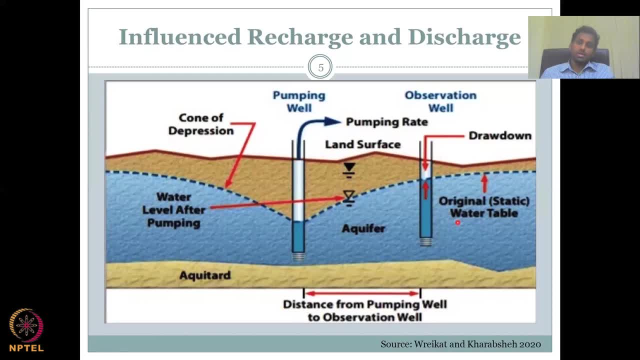 Because they put in a pump, they did not talk to others. they start sucking all the water out and causing the cone of depression And because of this there is an induced discharge. The water level comes down. That is a discharge. It is induced because of: 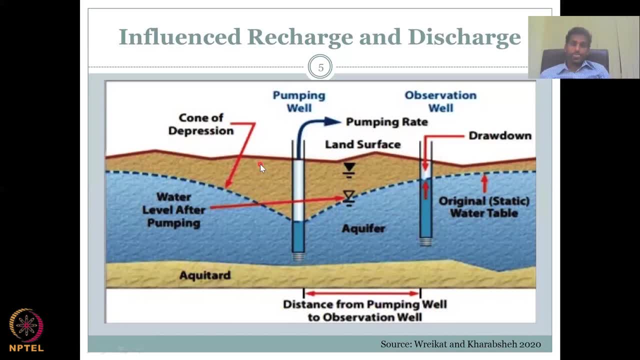 It is induced because of the pumping from a different well. Here we can say pumping in observation well, but hypothetically it could be two farmers nearby each other and pumping a lot. So think about even houses. You can have a flat system, an apartment, and right next to it a single house. 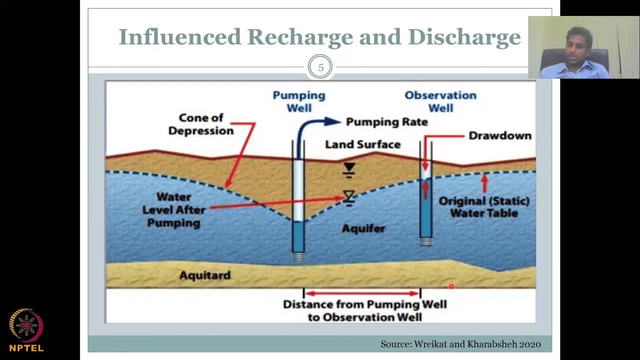 The single house can have a well and they can take water. Their need is very less. You know, maybe five people are using it for drinking, But the flat apartment's need is big. So if they pull too much water they would eventually pull the water off the neighbor also. 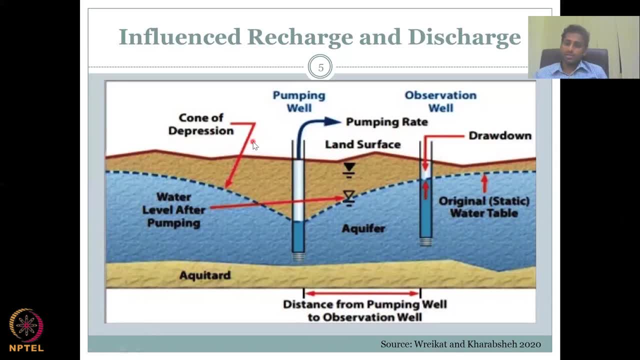 So this is the important part about induced discharge. What could be the induced recharge Same as you have water discharge being induced because of the pumping. If there is a recharge happening here, it would recharge more here because of the cone of depression. 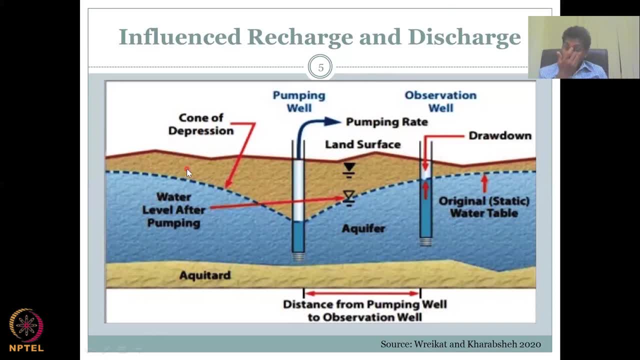 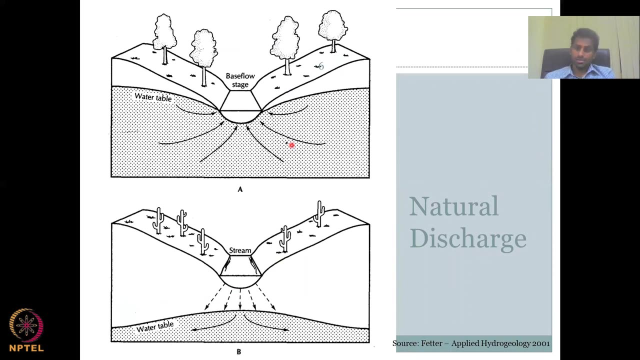 Why would water go into a place where there's high potential? It wants to go into the low potential And where there is more space. So because of this, pumping induced recharge can also happen. We also looked at the natural discharge and recharge, which is again we'll have to go through it because of the terms of recharge and discharge. 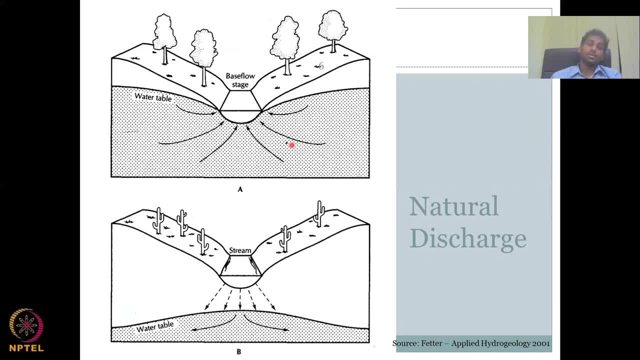 You have the gaining stream versus the losing stream. In the gaining stream, which is on the top, a river is flowing through a good forested area And the water table is at a much higher level Because of the forest. there's good soil. 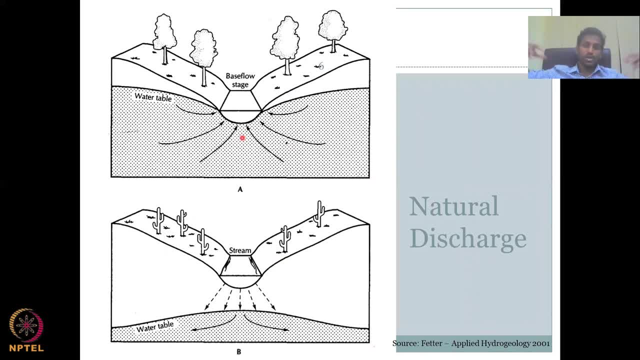 And good soil can have more water infiltrate and keep, And so the water level is high. It can come down into the stream, So that is a gaining river. The river gains, So that is a recharge from the groundwater. 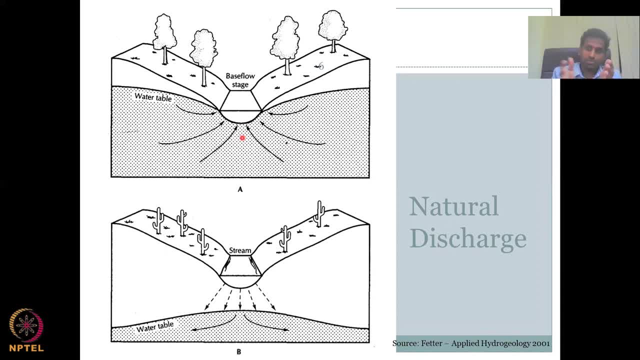 But the groundwater is discharging into the stream. As a stream, it is getting water, So it is recharged by the groundwater. As a groundwater. I'm losing my water to the stream, So the groundwater is discharging into the stream. 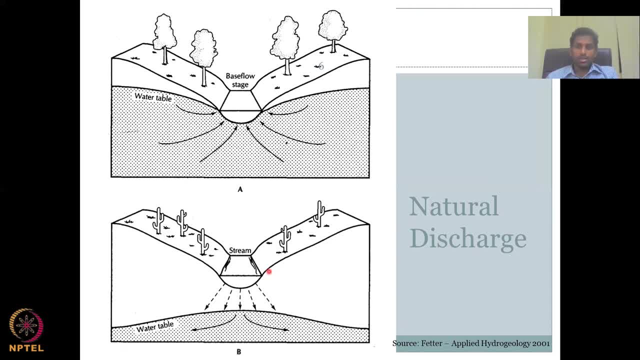 The other diagram where we saw a losing stream. here it is natural recharge, not discharge, Because groundwater is not going into the stream. On the other hand, the stream is giving water to the groundwater Because the stream is at a high potential compared to the groundwater, which is at a low potential. 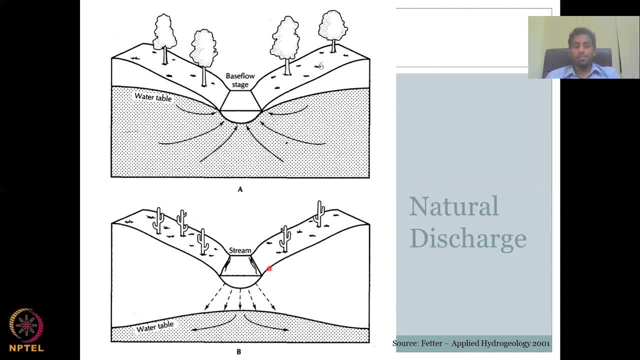 This act of getting more water by the groundwater, through the stream, through a losing stream, is natural recharge. So if you have pumps here, then it becomes induced. Here we are only talking about natural process. Once you put an engineered process inside, then a lot of induced processes can happen. 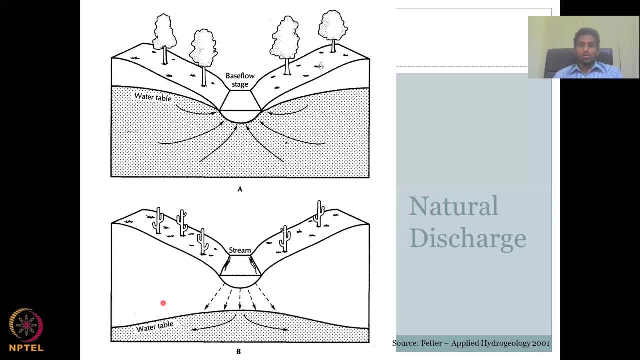 So with this lecture we have seen about the recharge and discharge mechanisms. We have seen the timeline that takes for these mechanisms Anywhere, starting from days to years in an unconfined unit, a consolidated unit which is much more down, deeper. 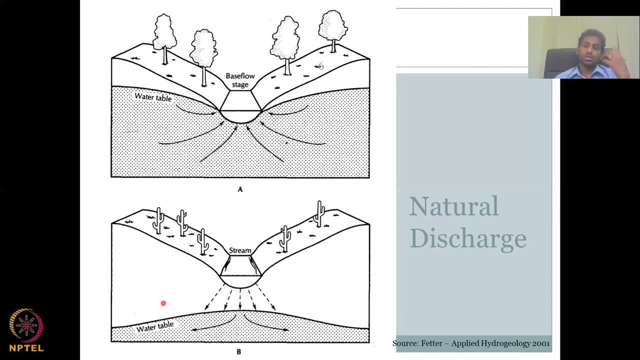 I'm talking about unconsolidated units or unsaturated units. Water can move within days to years, Whereas if you go beyond a confining unit, an impervious unit, then it can take years, multiple years, Centuries, and then, furthermore, another layer, impervious layer, can take you millennia. 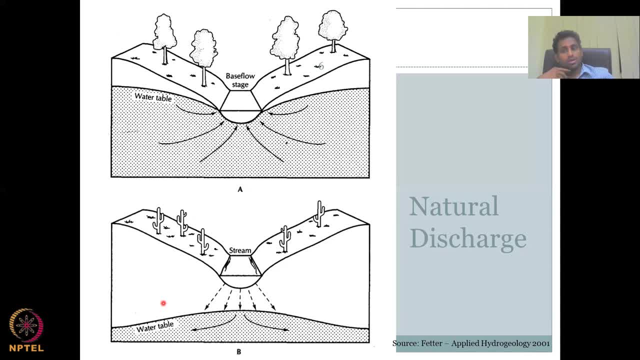 So it is kind of very important to understand the recharge process and the time it takes. It is a slow process because of the presence of sediments, rock and other materials. Once you know the recharge process, the time, as per say, then you could look at induced processes because of pumping. 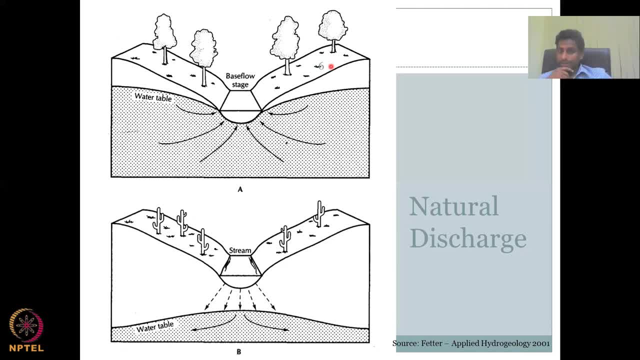 And induced discharge because of pumping. And also we saw that in this lecture- your groundwater, which you claim because you're putting your well and say, no, it is my water, It is not just your water but the water of the surrounding area also. 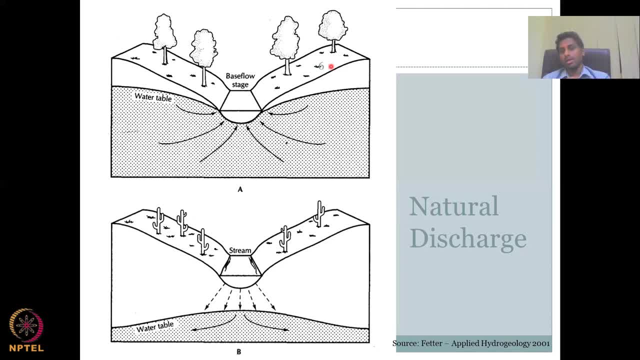 So just because I'm not putting a well in my field doesn't mean you can take my groundwater, Because groundwater is a communal source. Maybe the farmer did not have money, cannot afford it, And that is where, in the rural water resource management course, we'll be looking at how to pool farmers to better manage this resource. 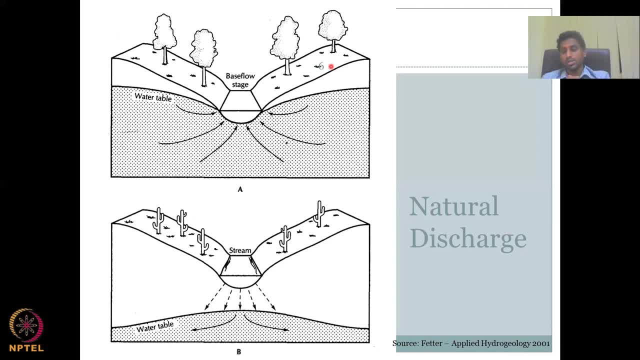 In one of my field works as a project scientist. we looked at mobilizing farmers, sensitizing them, saying: not all farmers can have pumps, Not all farmers can have tractors, So can we work together to conserve the groundwater, For example, if seven farmers say okay? 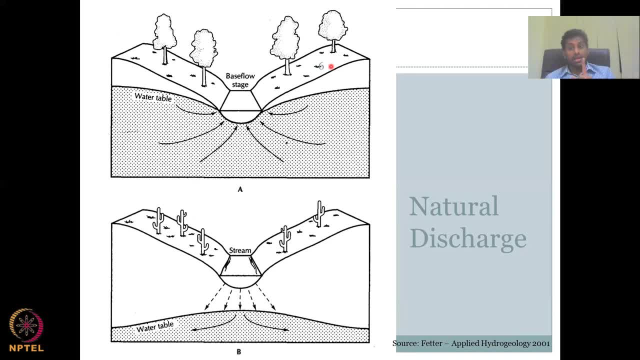 You take the groundwater, I won't manage my land. I will not manage my land. I put cement on my land. Will the other three get groundwater? They won't Because he or she has to give the land for recharge. Okay. 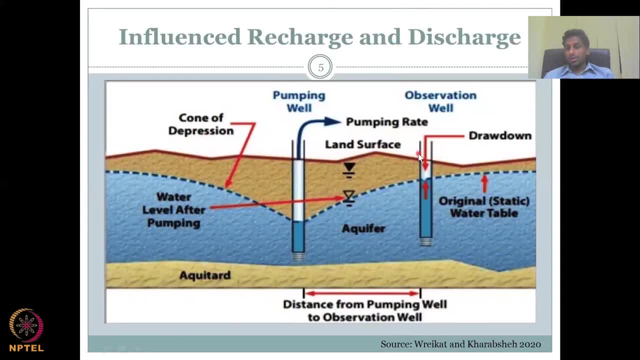 So that is very important Again here: If this farmer is not pumping, but still he's recharging the groundwater. So this farmer, which is farmer A, is taking all the water from farmer B And his hard work, his or her hard work.